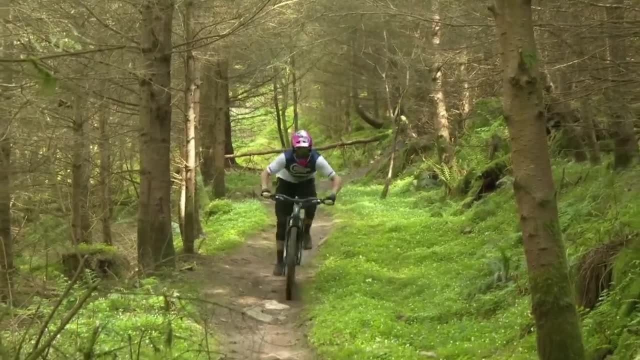 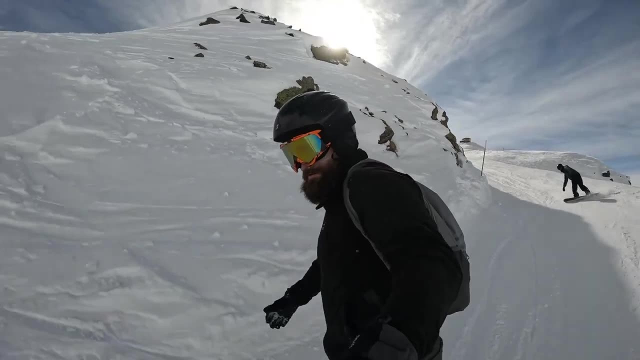 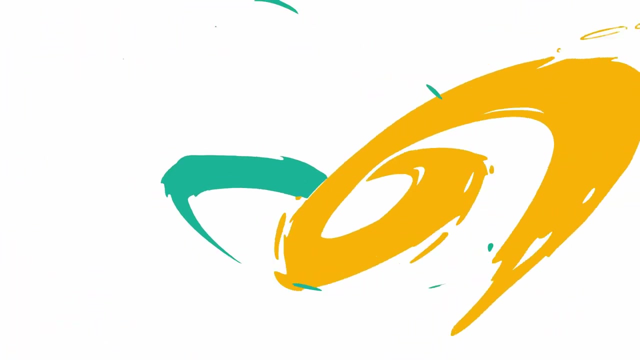 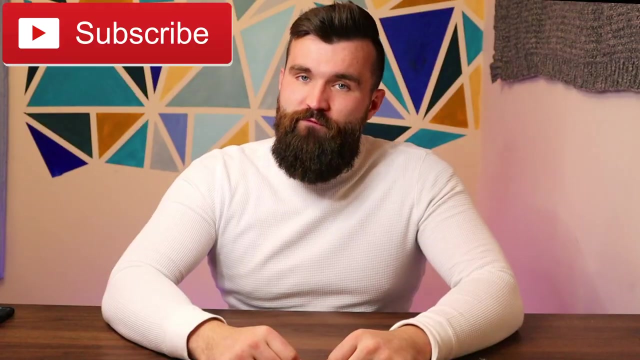 What's up? it's me, Mr Radley, and today we're learning about friction. What's up, guys? it's me, Mr Radley, and today we're learning about a force called friction. But before we begin, hit that subscribe button and the bell notification button and get ready. 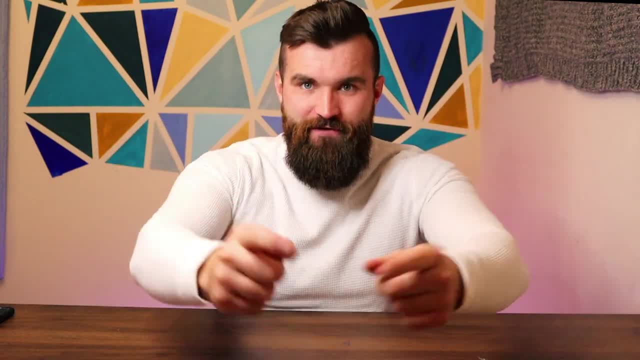 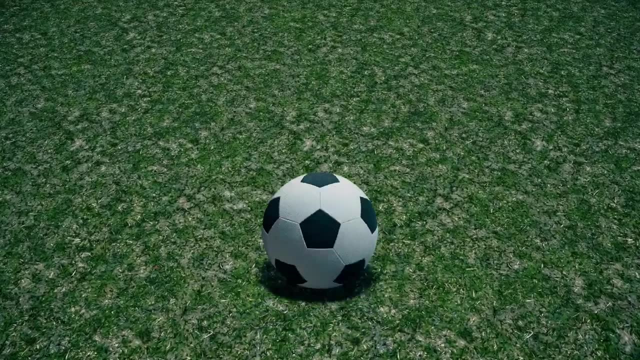 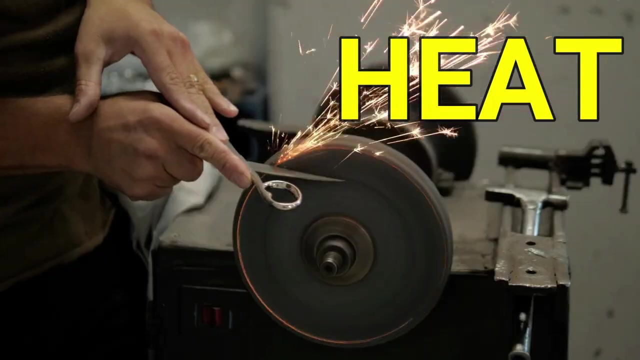 to do the starter questions on your screen right now. Friction is a force that opposes movement. It's the whole reason that a ball rolling down a hill will eventually come to a stop. Friction occurs when two surfaces rub against each other, and when they do this, they produce heat. If you don't believe me, try rubbing. 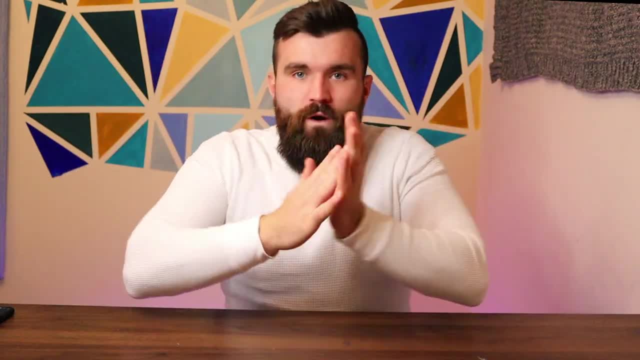 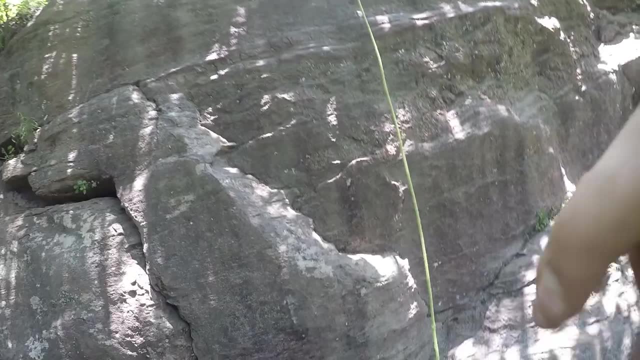 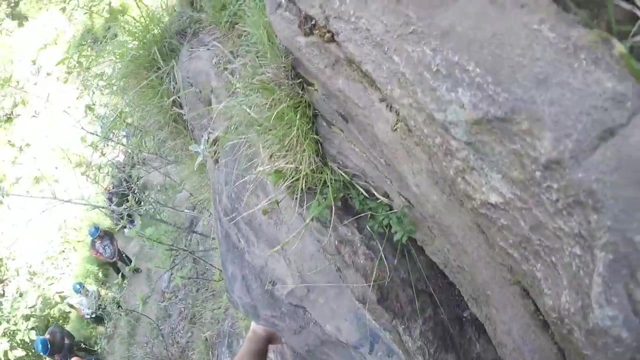 your hands together and you will feel the heat. Ouch, Whatever direction one surface is trying to move, friction will pull in the opposite direction. For example, when I'm rock climbing, the surfaces of my hands are pulling downwards thanks to gravity, But friction will be pulling upwards. 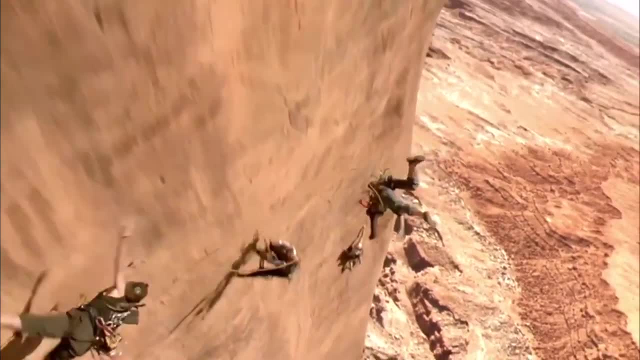 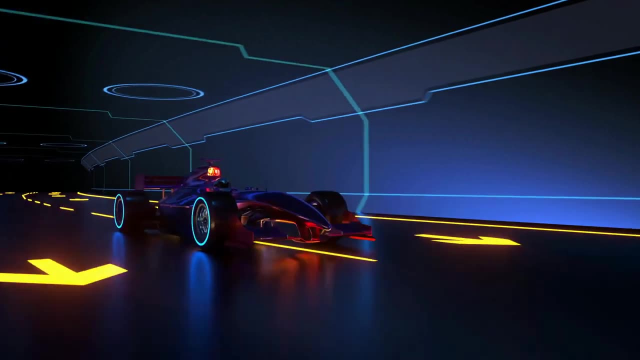 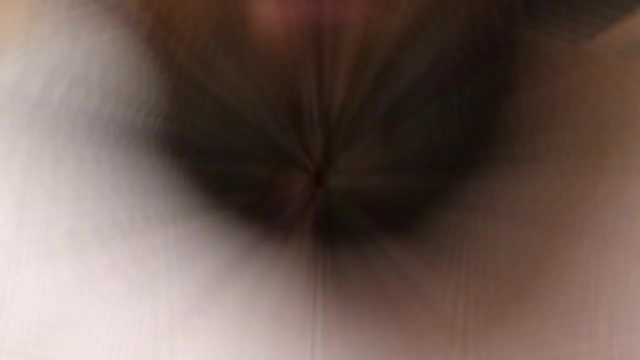 And preventing me from falling to my death. Wow, thanks, a lot friction, A lot of the time. more friction is useful because it stops things from slipping, Like when we are driving, rock climbing or even mountain biking, And one person who knows all about this is my friend, Keelan Grant. 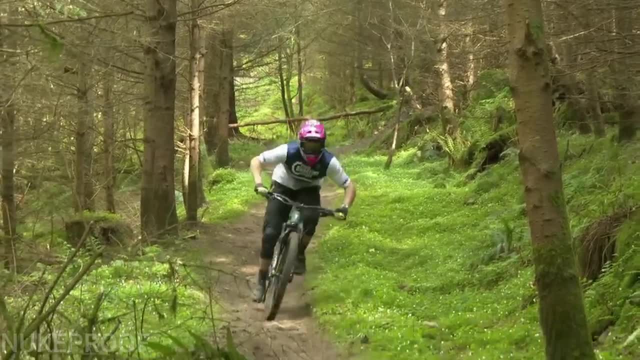 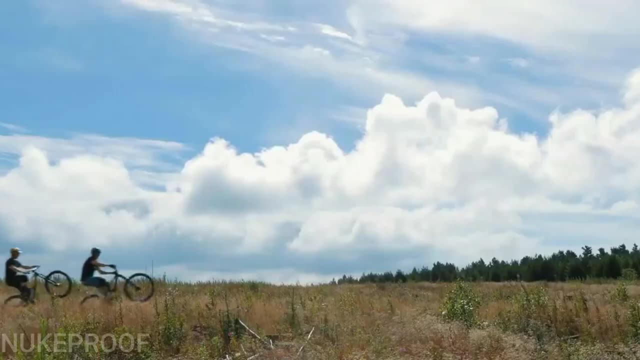 Hi guys, it's Keelan Grant here. I'm a professional mountain biker and today we are going to talk about friction. First of all, friction is one of the things that we want to discuss with you all. Right now, we are in our own mountain road. We have a lot of pressure on our hands. 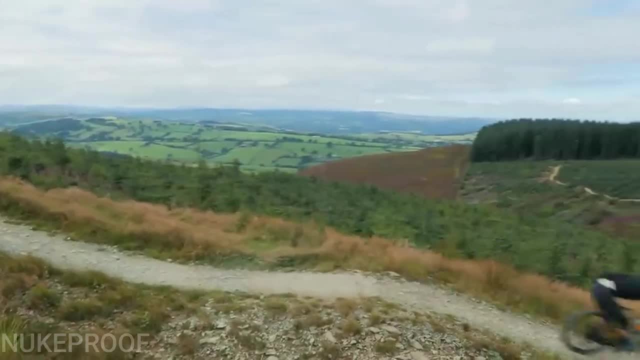 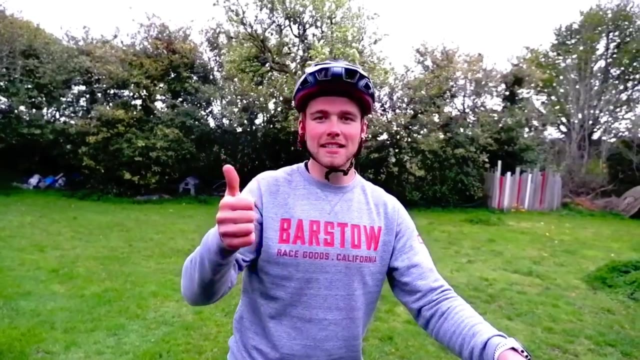 We are all quite exhausted. I don't think we have any additional energy, So we need to build up our muscles and start to improve on the stretch. So we need to keep the muscles and the muscles in good shape. Hi guys, it's Keelan Grant here. I'm professional mountain biker and today we are going to talk about friction. 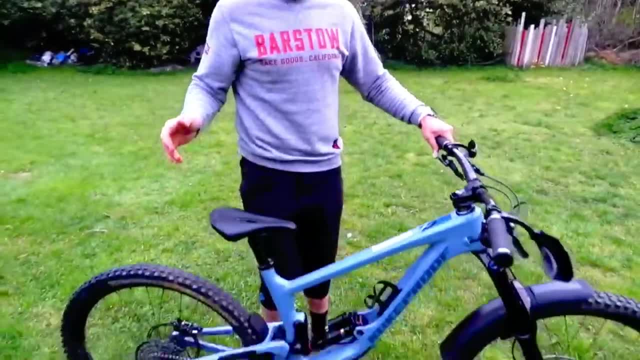 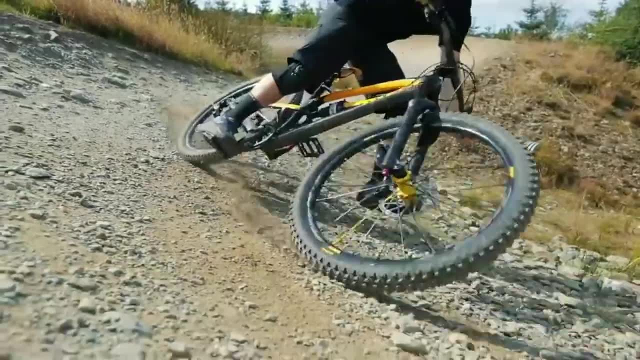 So first of all there is this Bilobo to the side. I did a lot of mountain biking and for them, a lot of exercise, so they definitely took out a lot of time. My bike- here we've got my tires, The first contact point with the ground. this allows me to slow down better and also cut into the ground so I can maneuver sharp turns better. 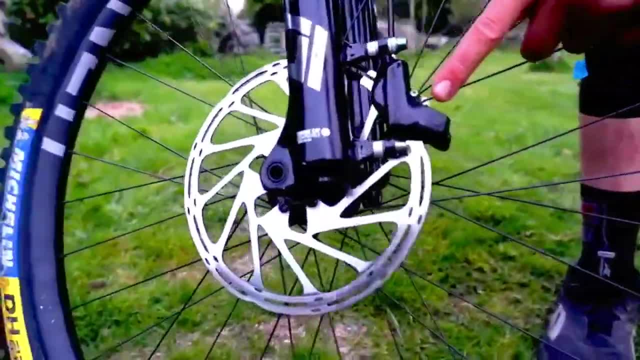 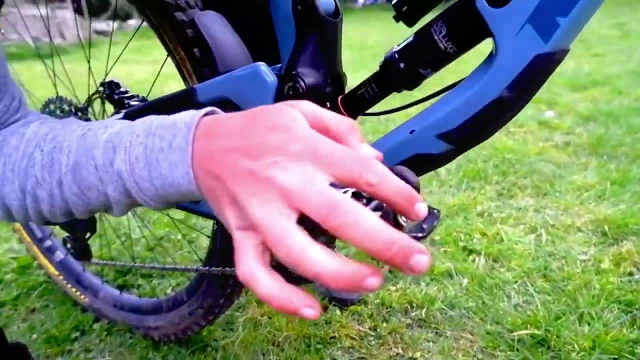 Also on my bike I've got some brakes. These are a pad and a disc that push together, and when pulling these with force, this helps me to slow down as well. As you can see on these pedals, sharp pins that allow these to stick into my shoe. This also creates friction to help my feet stay on the pedal. 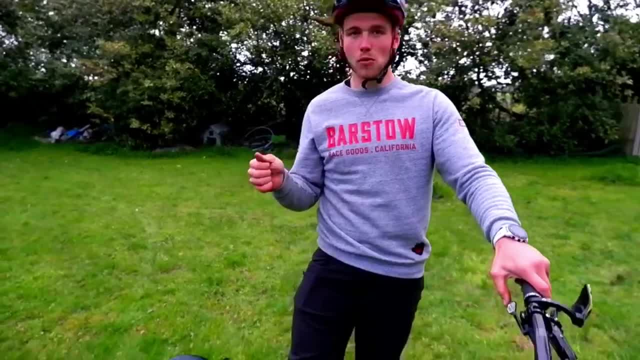 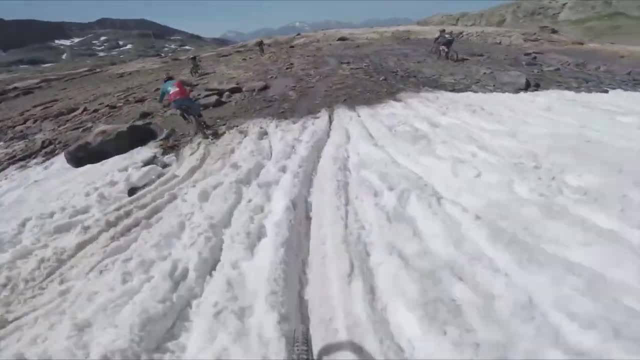 So these are all the points of friction on my mountain bike. Normally in the dry there is more friction created. The bike is easier to turn and slow down. Conditions are wet, being even icy. Less friction means the bike is harder to slow down and harder to maneuver. 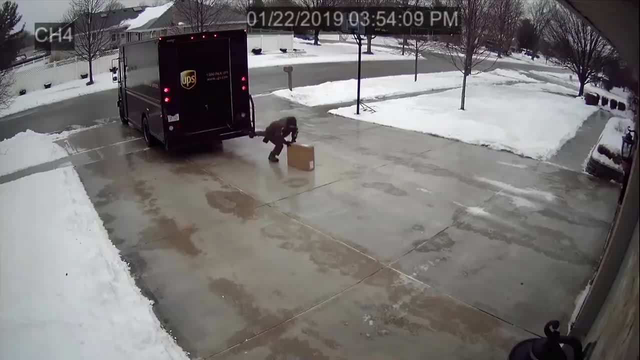 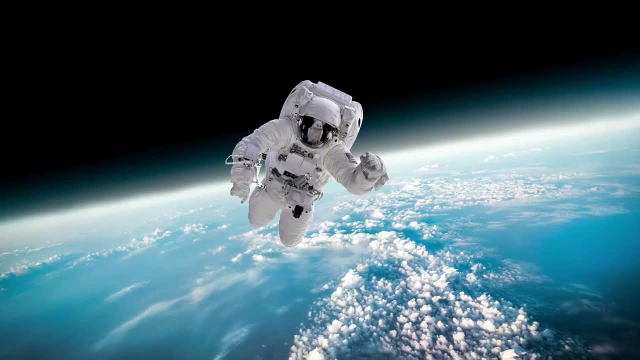 Alright, Mr Bradley, back to you. In a world without friction, we would have no control of where we were going and we would not be able to stop, Just like in space. In outer space, things never stop moving, and that's entirely because there is no friction. 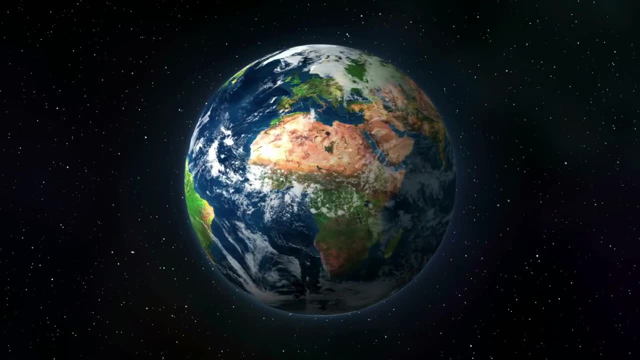 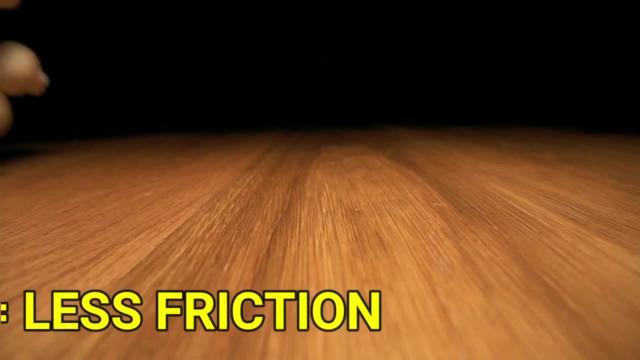 Even right now, Usually the planet that we are on is moving through space. Things that have rough surfaces have actually got more friction and will stop moving things more dramatically, While things that are a little bit smoother have less friction and will not stop things from moving as quickly. 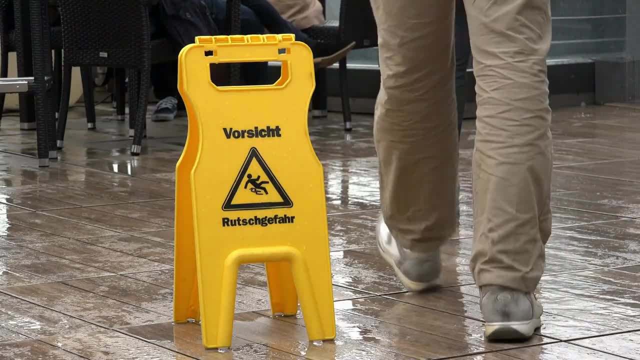 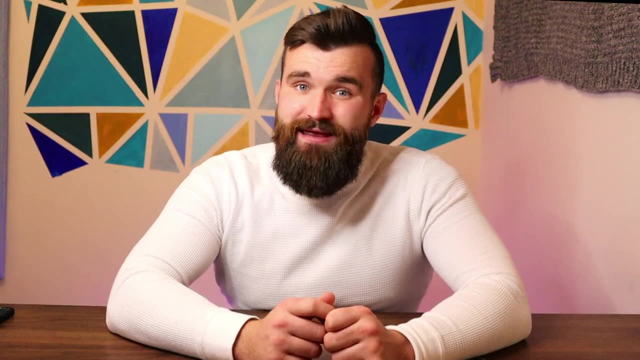 If a surface is covered in water, it will actually reduce the friction greatly. The reason for this is the water will fill in all of those bumps and lumps and can move freely across the surface, Meaning it will have a lot less friction. No friction can be a problem. 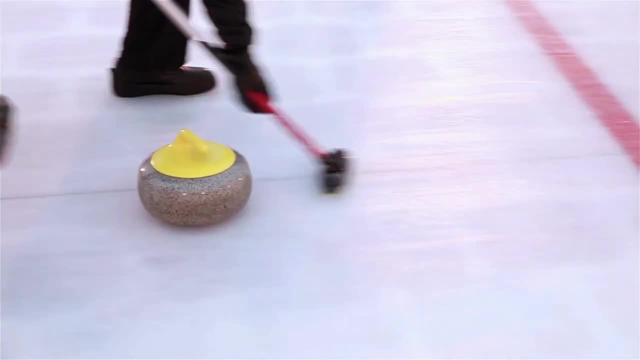 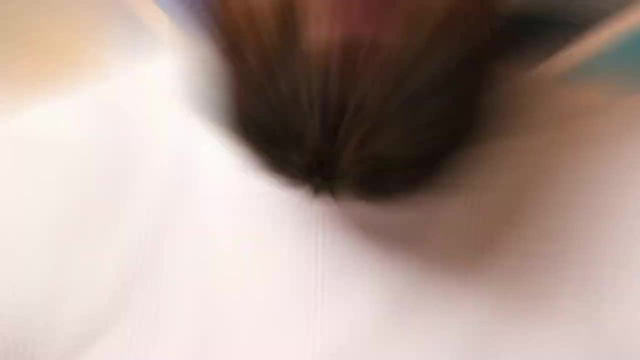 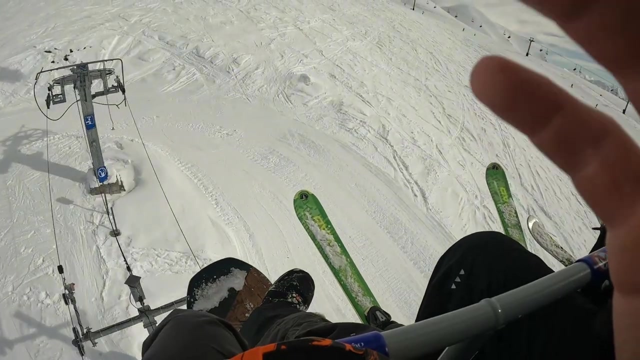 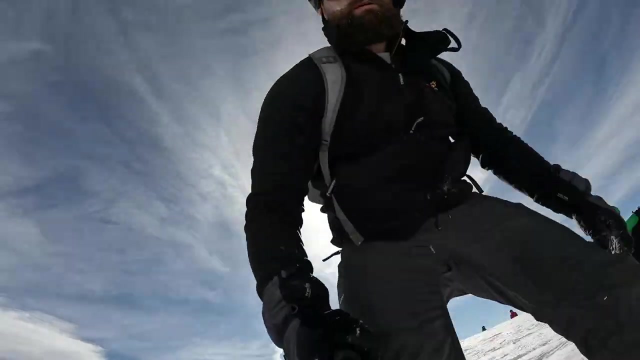 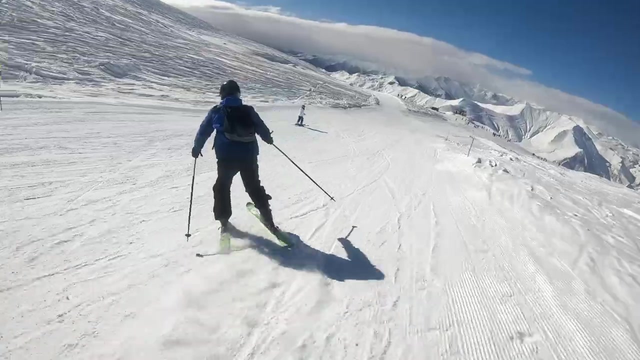 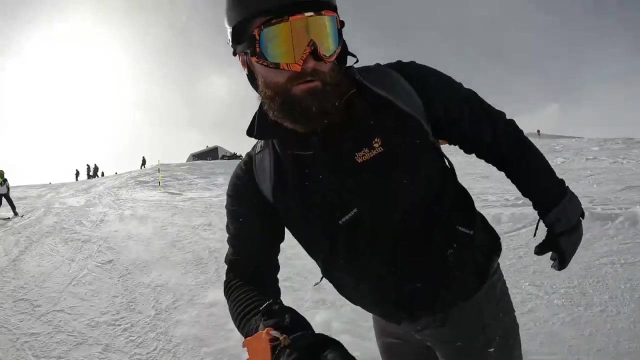 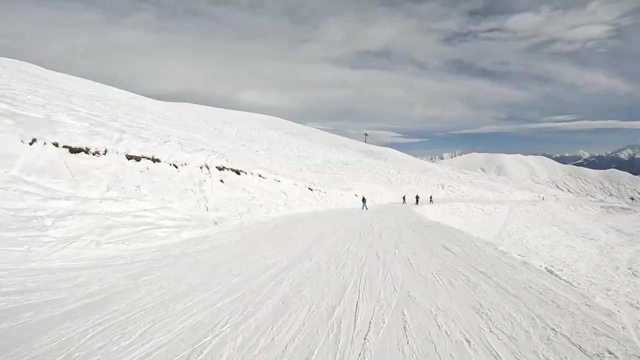 But still, sometimes less friction is actually a good thing. Low friction allows us to do a lot of cool, fun things like water slides, ice skating and snowboarding. When you do all those things, you can have a lot of fun. I really like the effect of the water on the surface. 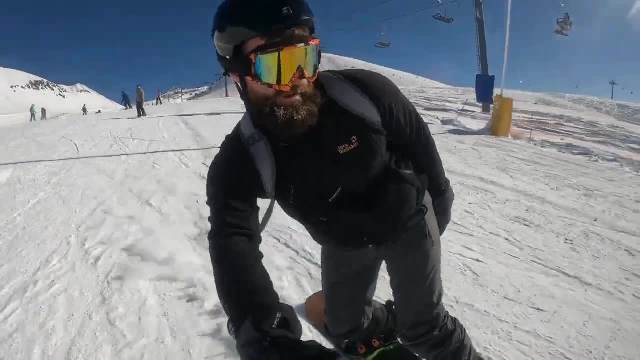 You can almost not see the surface. The surface is kind ofλο, not so smooth. You can see the metal surface- A lot less friction. That's the difference. It's not as good as the surface. You can see the metal surface. 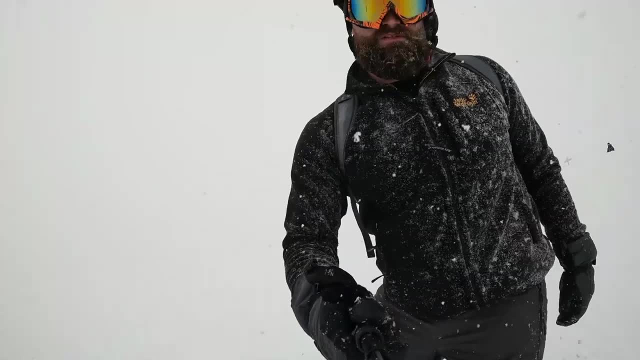 Nothing is going to be as smooth as the surface. That's the difference. That's it. If we've got a lot of friction going on, then that's where the curves come in And that's where the air comes in. That's the difference.